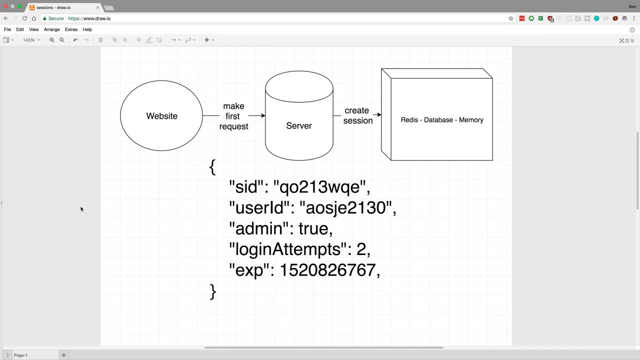 Hey guys, I wanted to go over how sessions work in a web server, And I'm going to be going over one way that's very common and that works really well, But there's other ways to do it as well. So, if you're not aware, sessions is just like a piece of data that a server keeps track of of a user as they're using the website, And this can be very helpful because you want to keep track of what the user has done before. 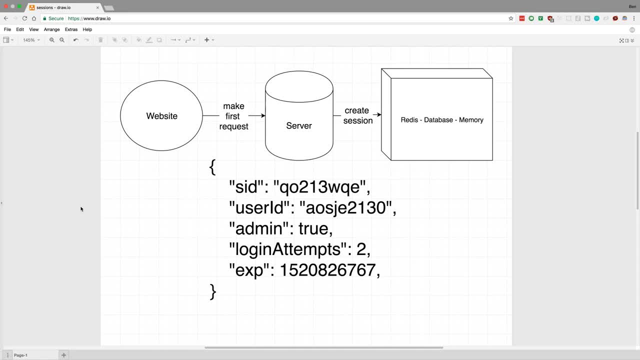 And what they've done on your website so far. So it's a way of keeping track of what they've done And this is how it works. So let's say you're on a website and you make a request, This might be the first request you make, or maybe you've just logged in, going to go to the server and then the server is going to create a session, And so when I say they're creating a session, what that means is they're going to be creating an ID And 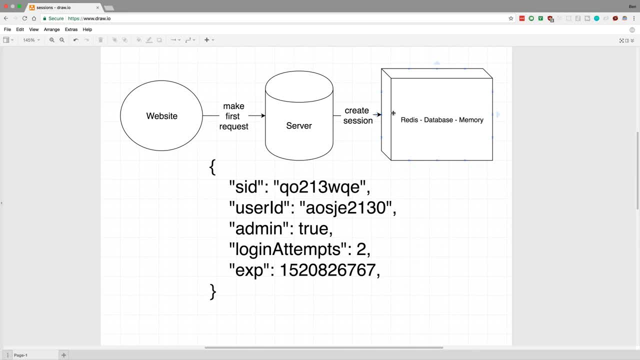 storing this in maybe a Redis or a database or just in memory. And what I mean just in memory, that might be just like a object where they're storing a whole bunch of sessions or a long array, something like that. That's just in the memory of the server as opposed to like a database or Redis. So, for example, I have a little piece of sample data here. this might be like what looks a session, might look like some data. 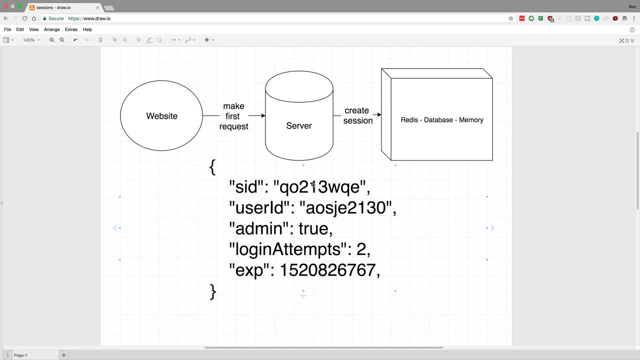 So this thing up here is the session ID Sid, And so to create a session ID, what you would do is generate a Sid like this. So session ID is just a random string, could be a UUID, which is probably recommended, And if you don't know what that is, that's just a good way of creating an ID, because it's a random string with some specific attributes of how it's made. But, yeah, so it creates an ID And at first you don't have any data whatsoever in your 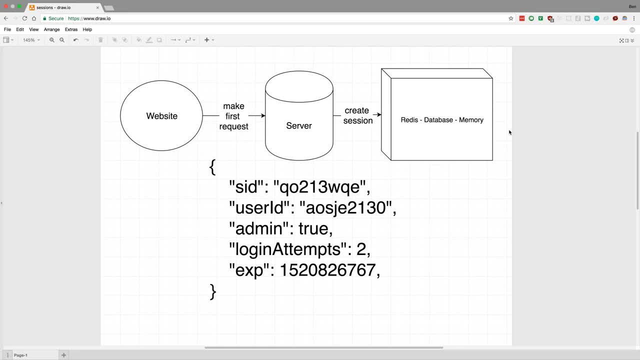 session. Now they're making the first request. you might be able to store something from it, But most of the time, what you're going to do is you're going to send that ID back to the website And the website is going to store that ID in some way. maybe they're going to store it in cookies, local storage, session storage, pretty much it doesn't matter. Well, it does matter, But they're storing it in some place where it's persisted, And what I mean by that is when the user refreshes the 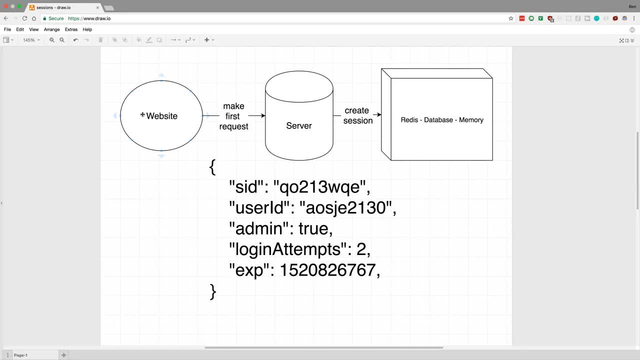 page or leaves the site and comes back, they have that, that ID still associated with them, And then, every time the user makes a request, the server will look and see whether this ID is stored and whatever they're using to store it. And so what this allows you to do is, when the user is making requests and doing stuff on your website, is to gradually add data. So the session is just a basically JSON. 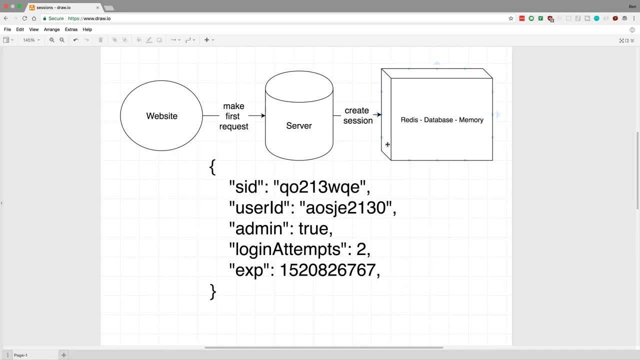 object. There's other ways to do it, But like this, where you just have the session ID and then any other data you want to keep track of. So as the user is browsing the site and making requests, you slowly generate more data. or you can generate more data And you can also generate, for example, an expiration date. So maybe after seven days or five days there it's expired. in this they get a new session. 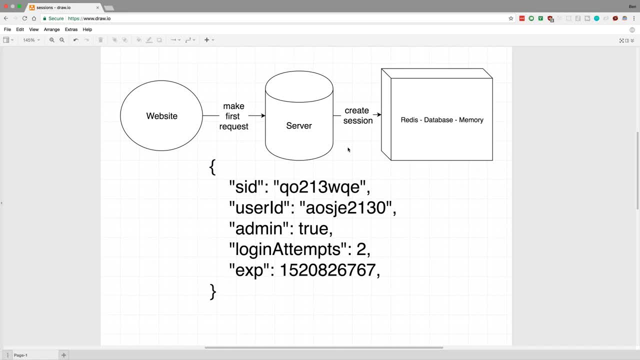 And the data gets old or whatever. So some use cases for this are keeping track of whether the user is logged in or not. So right here I have the user ID, So I know who the user is after they log in and I can store that as the user ID, And I might want to store also some metadata, So whether they're an admin, but you can also use this for pretty much any kind of tracking you want to do. So one thing you might want to do is